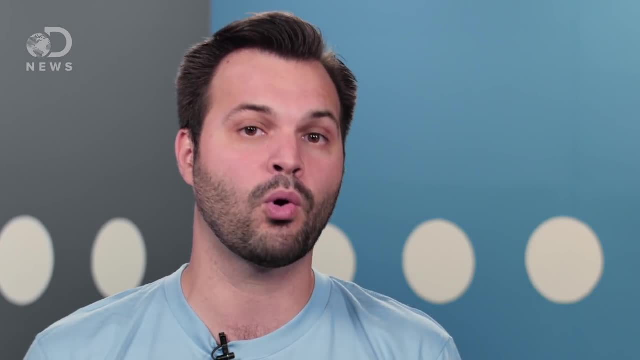 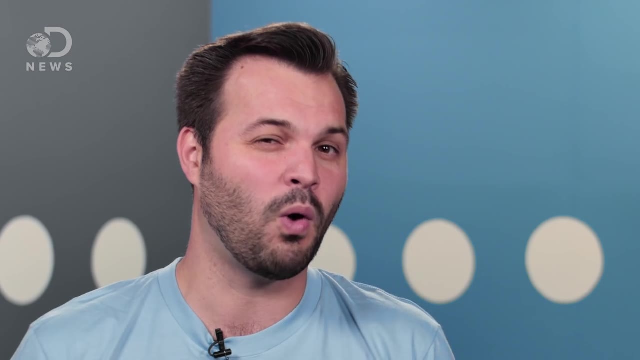 having never been diagnosed. This research shows white men are more prone to depression stemming from stressful life events than black men or all women, Although more research is needed on why this is. In a 1995 study in Progress in Brain Research, they looked at the brains of those who committed. 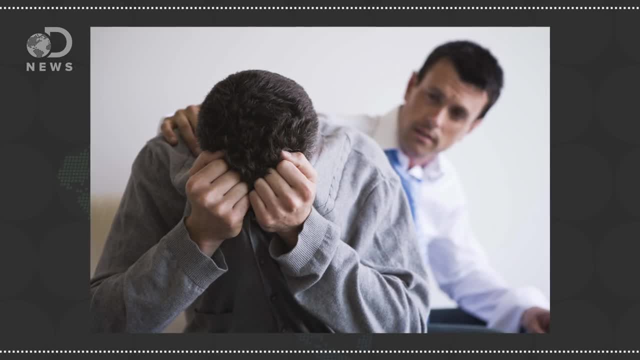 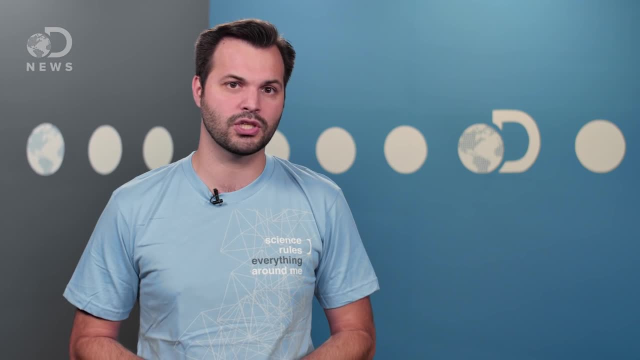 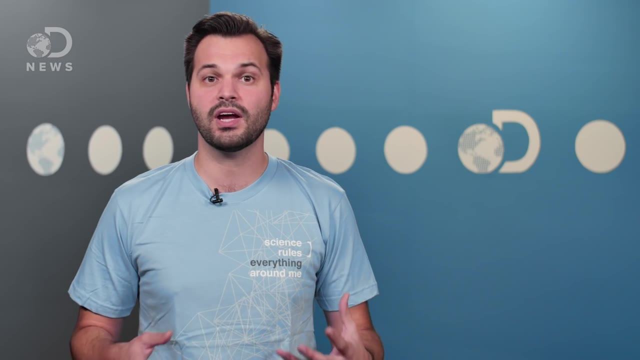 suicide and compared them to the brains of people who hadn't. All of the subjects had depression, Even though both brains had lower levels of serotonin activity due to the depression. those depressed people who'd contemplated suicide had different or different levels of orbital cortices than those who hadn't. 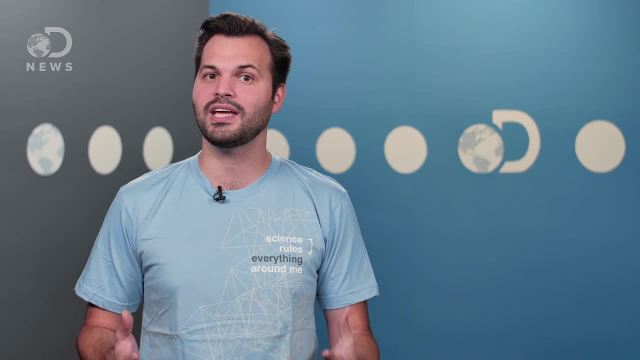 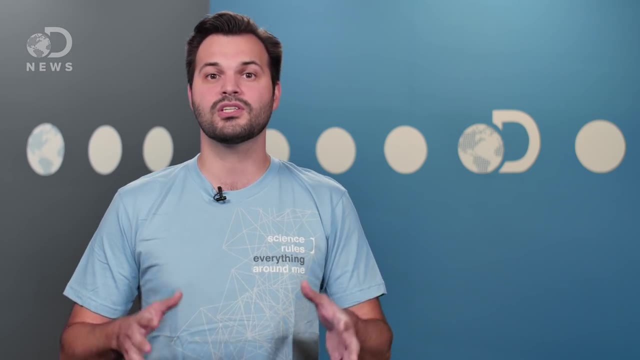 Those areas are connected to executive function, decision-making and behavioral inhibitions. The researchers said most don't think of suicide at all, while others think of it first because suicide victims often have trouble controlling impulses, Which brings us back to firearms. 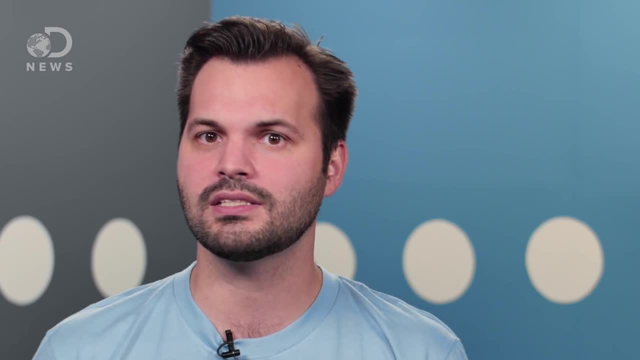 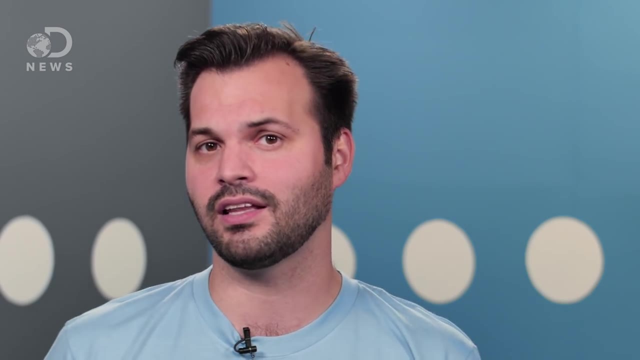 Firearms facilitate impulsive actions. Papers in the journal Crisis and Suicide and Life-Threatening Behavior found suicides are commonly impulse-driven, not elaborately planned like you would see in television and film. In fact, according to their findings, 25 percent of suicide 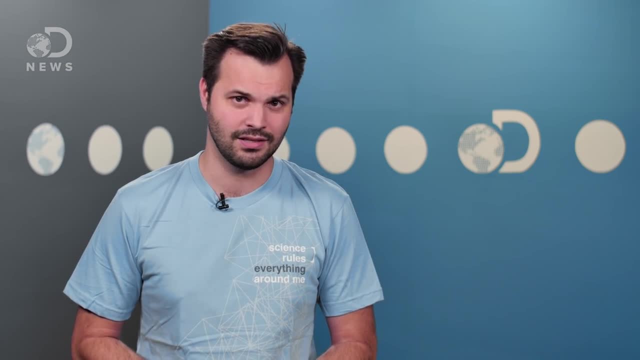 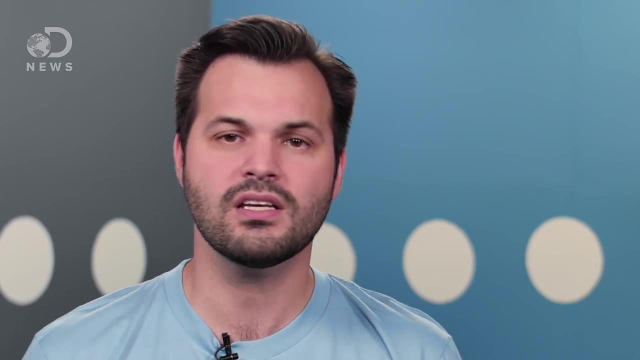 attempters said they deliberated for less than five minutes. In fact, most- 75 percent- debate less than an hour and only 13 percent thought about it for more than a day. Because guns are point-and-click, it stands to reason when depressed men making an impulsive 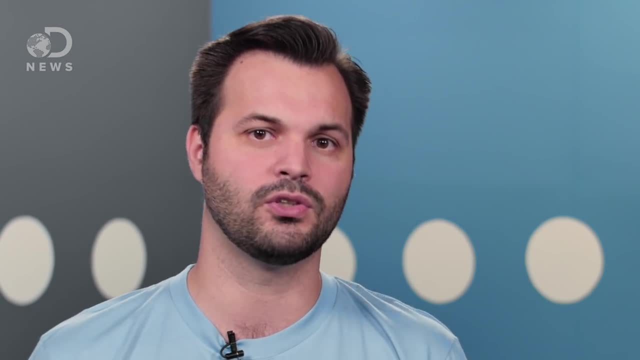 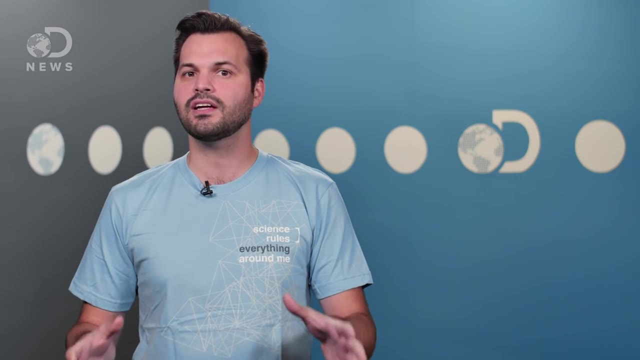 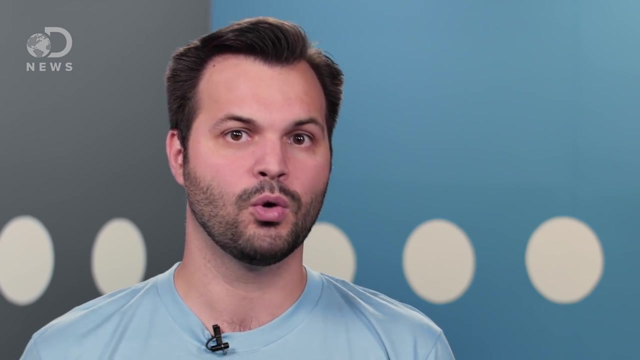 action like suicide can reach for a gun. that's what they'll do. The Harvard Health Policy Review looked at academic literature connecting suicide and access to firearms. Having a gun slightly increases suicide risks overall, and the journal Trauma found rates of suicide in states with the most gun ownership was twice that of states with least gun ownership. 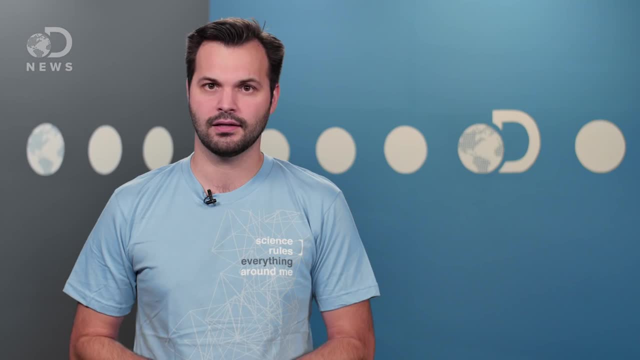 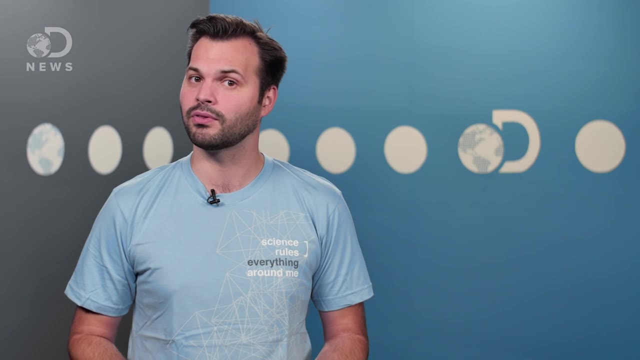 More guns means more gun-involved suicide by a lot. On top of that, according to a Pew Research Center study, men owned three times the number of guns, while whites owned more than double the number of blacks and three times that of Hispanics. 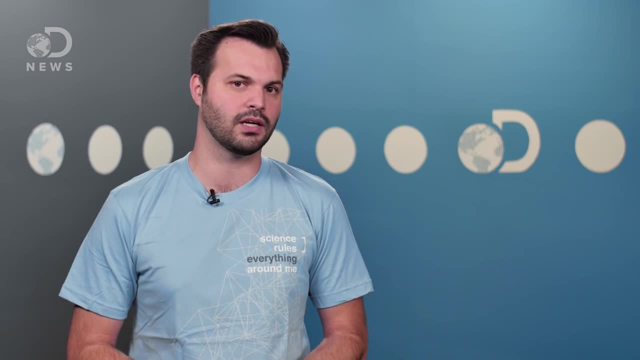 It would seem, the reason white men are eight times more likely to commit suicide with a gun is because they're depressed, have no control over their lives and are more likely to commit suicide with a gun. They have no way to deal with it, have a gun in their home and have decided to use it.